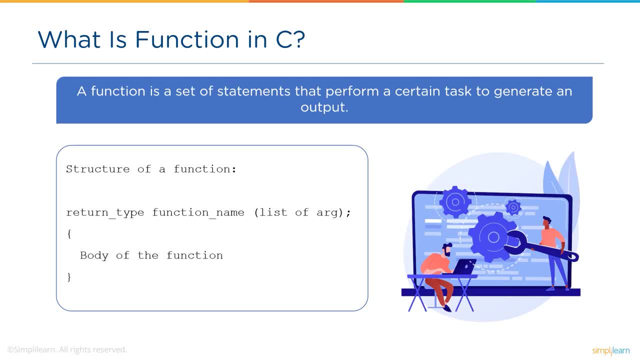 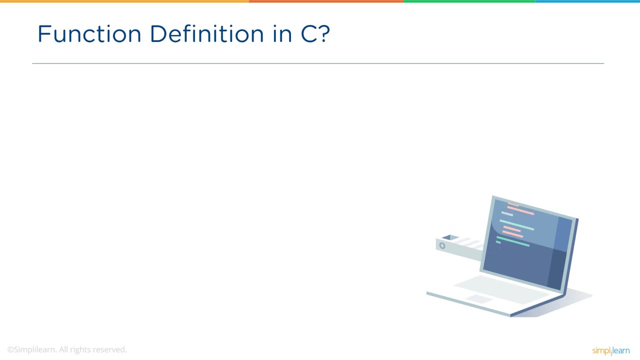 Now let's look at the structure of a function. In a function header we have return, type, function name and a list of arguments And the body of a function inside the curly brackets. Now let's have a look at the function definition in C In the given below, function definition. 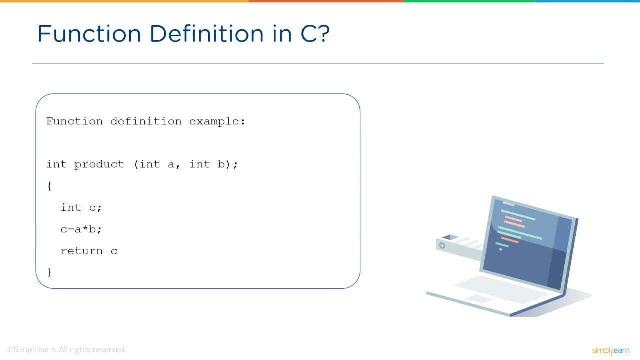 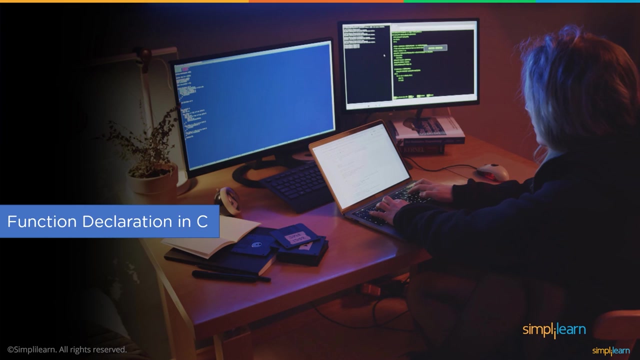 example, we have int as a datatype, product as a function name, followed by parameters a and b. Next, the body of a function consists set of statements to perform certain operation. So in this particular example, we gonna perform a product of two numbers. 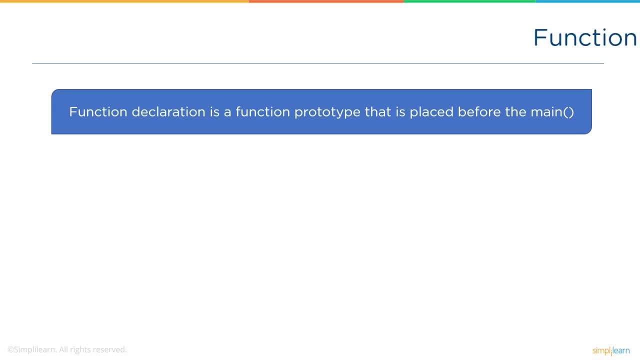 Up next we have function declaration in C. A function declaration is also known as a function prototype in C. There are some important things to know about function declaration, And the first thing is that the function prototype must be placed before the main function, And if the function definition is placed before the main function, then the 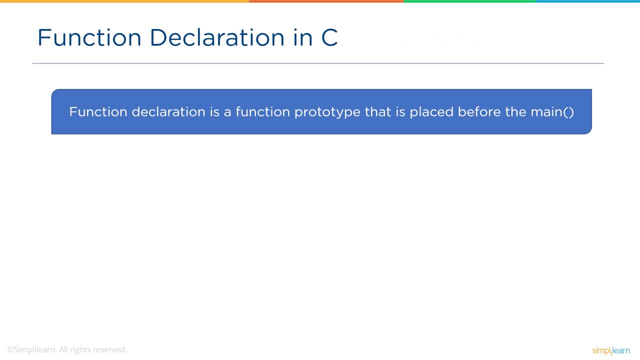 function prototype is unnecessary in the program. Next, function declaration may or may not contain parameters, Rather it may have only datatypes of variables. Then the function header must match the function declaration. Syntax of a function declaration is return type. 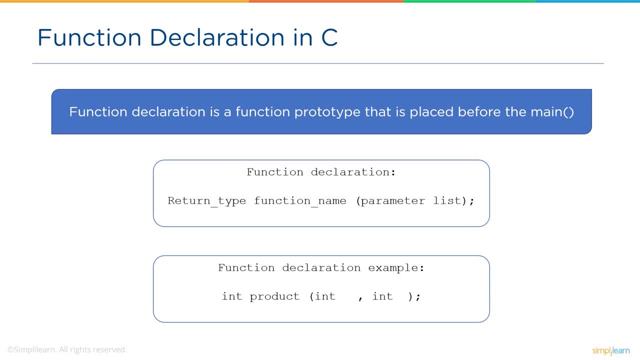 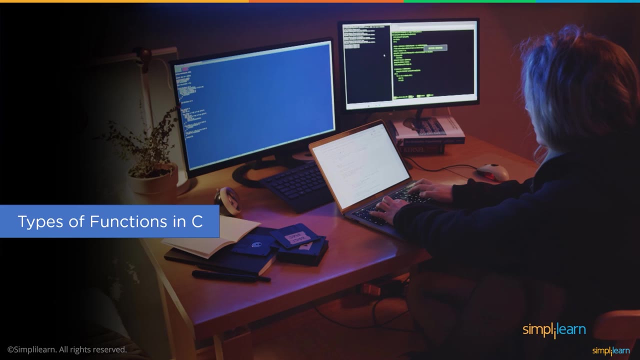 Name and parameter list, For example, int, product and datatypes. If required, we can also specify variables along with the datatype, like int a, int b. Now that we know function definition and declaration in C language, let's go ahead and understand. 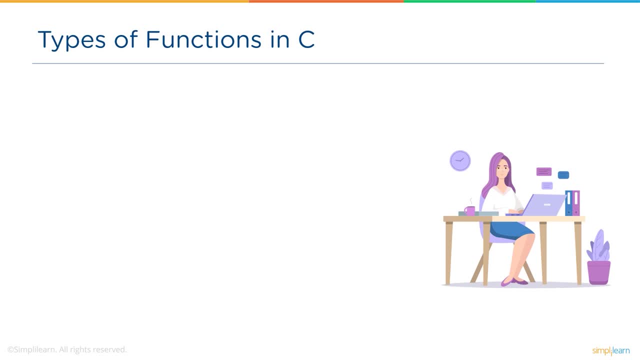 the types of functions in C. C has two types of functions, and they are library functions and user-defined functions. Library functions are built-in functions or we can also say predefined functions in the header file, For example functions like square root string. 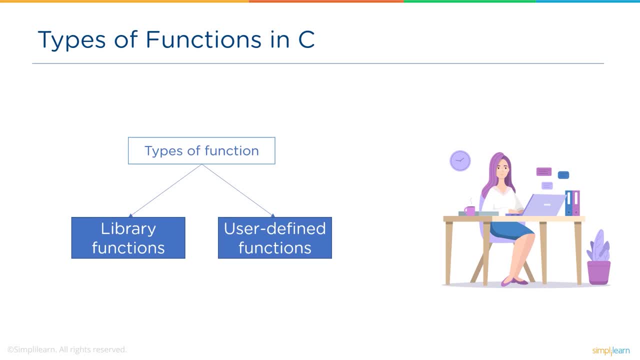 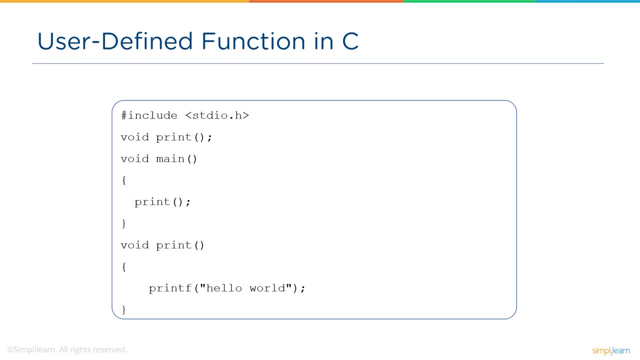 length, printf, scanf, etc. are predefined functions in C. To use library functions in the C program we include a header file corresponding to that function. Functions that the user defines are called user-defined functions. Let's consider the below given example. We 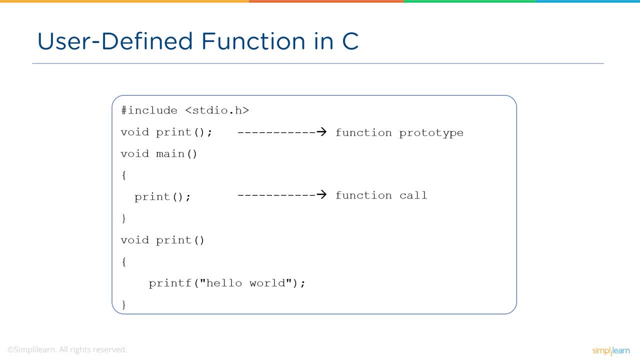 have three important features. The first one is the user-defined function. The second one is the function-prototype. The third one is the function-call. The fourth one is the function-def. A function prototype is declared before the main function. Next calling a function is: 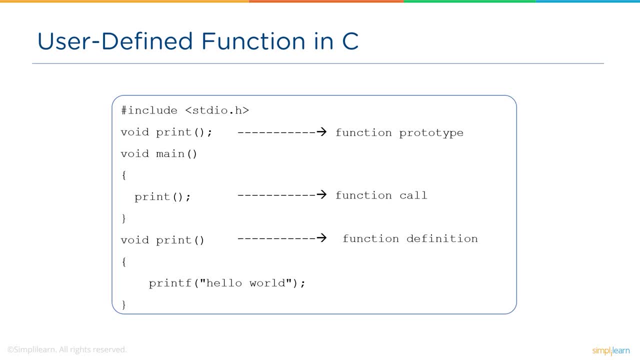 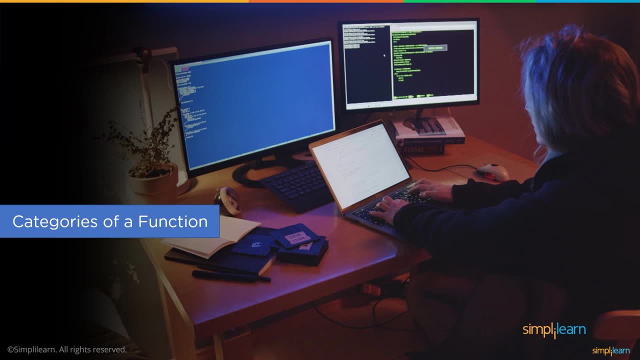 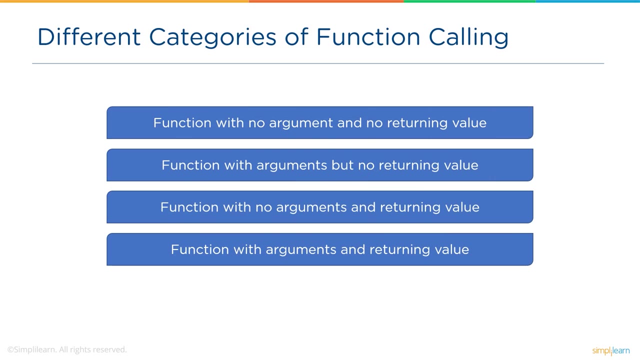 done inside the main function. And then comes the function definition, in which we have a set of statements to be executed. Let's now look at some different categories of functions in C: Functions with no argument and no returning value. Next, functions with arguments but no returning value. 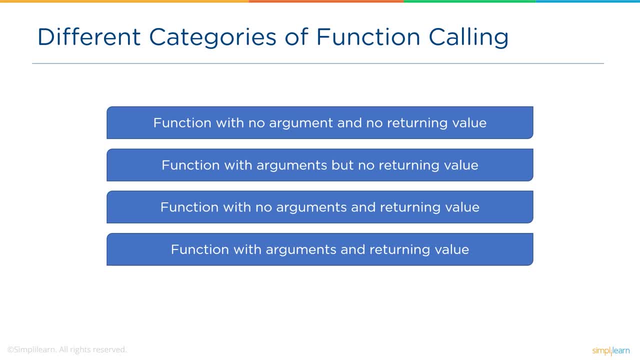 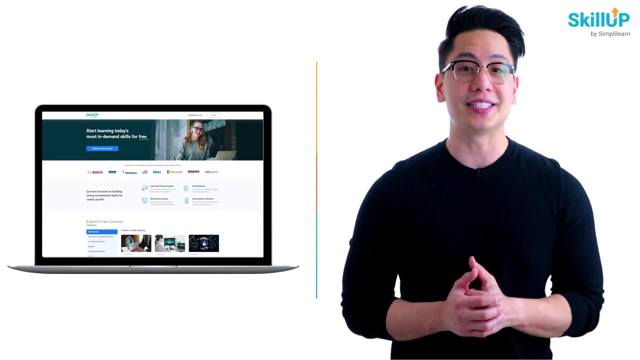 Then functions with no argument and returning value. And last functions with arguments and returning value. Let us understand them with the help of our programs. If getting your learning started is half the battle, what if you could do that for free? Visit SkillUp by SimplyLearn. 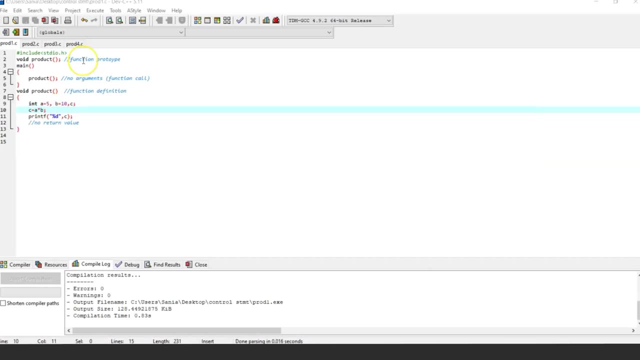 Click on the link in the description to know more. So this program is function with no argument and no return value. As you can see, we have declared function prototype, function call and function definition, In which we have function with no argument and no return value. 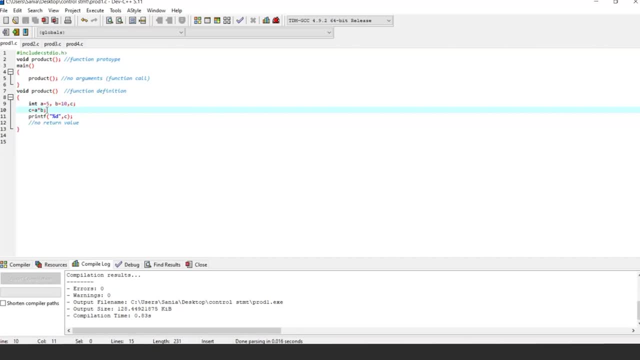 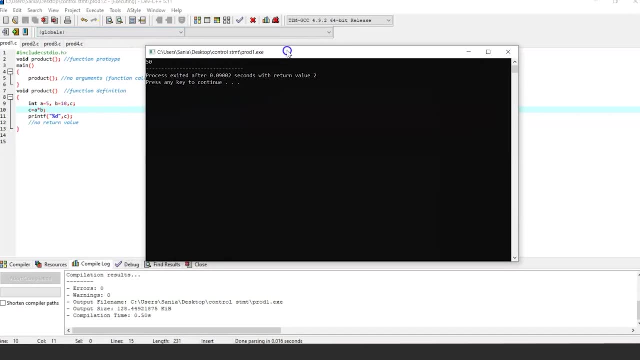 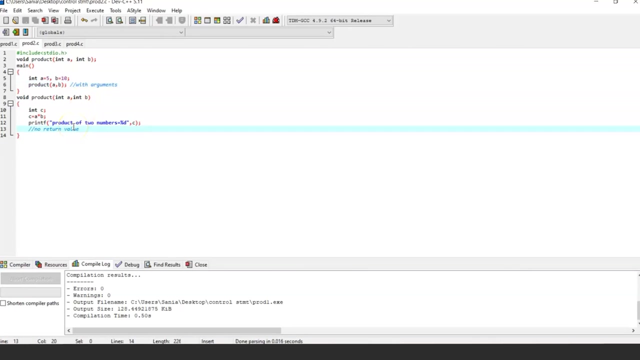 And we are going to perform multiplication operation using user-defined function. Now let's run the program According to the values of a variable: 5 and 10, we got an output: 5 into 10 is equal to 15.. Now let's run the program using a function with arguments and no return value. 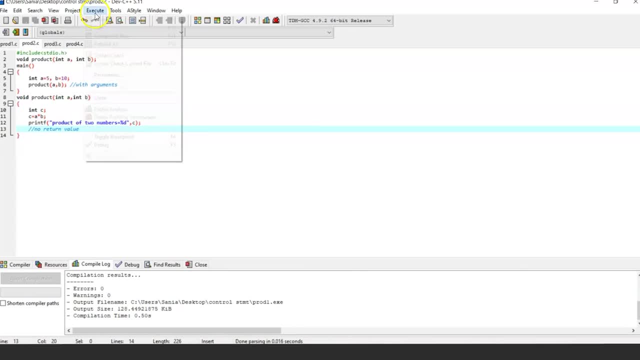 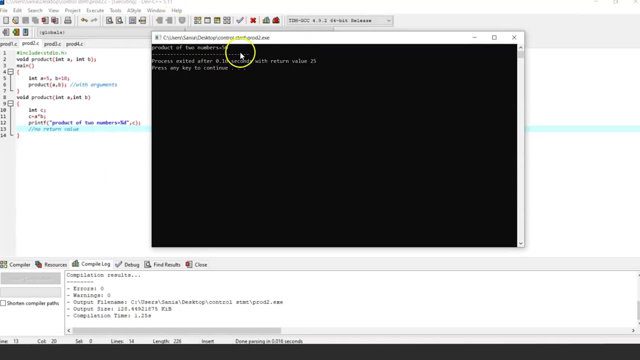 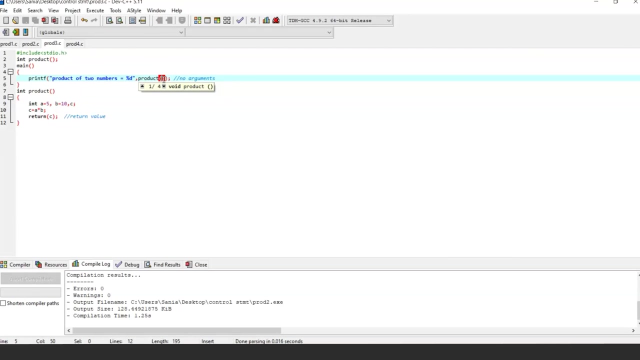 And let's perform the same operation, that is, multiplication. As you can see, product of two numbers is equal to 50 and we got an output. Next program is using a function with no argument and with return value. To get a return value we have a data type, int. 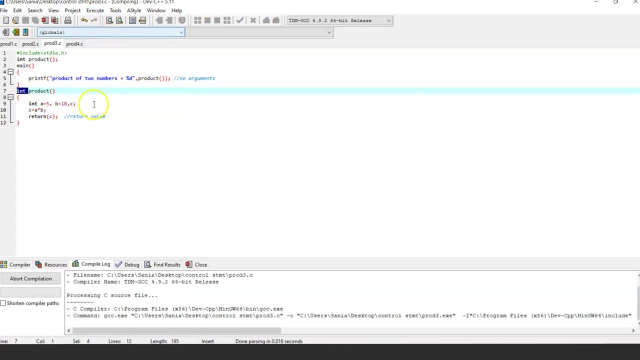 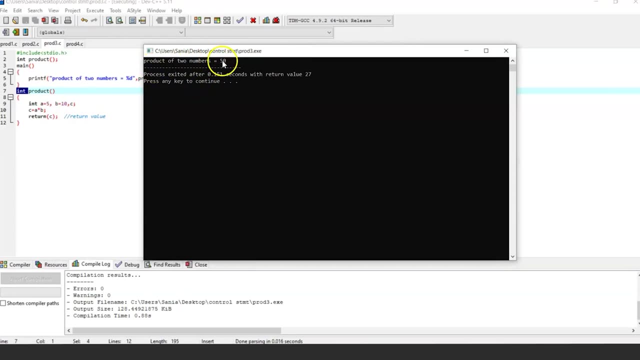 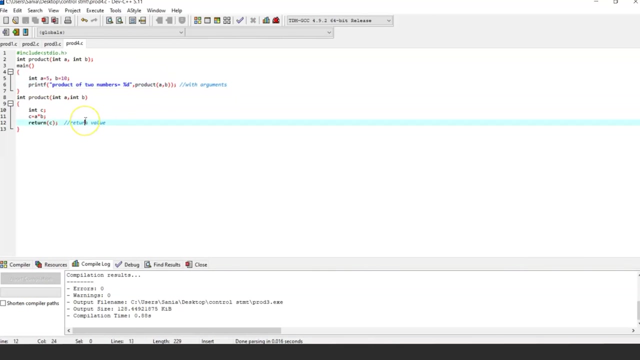 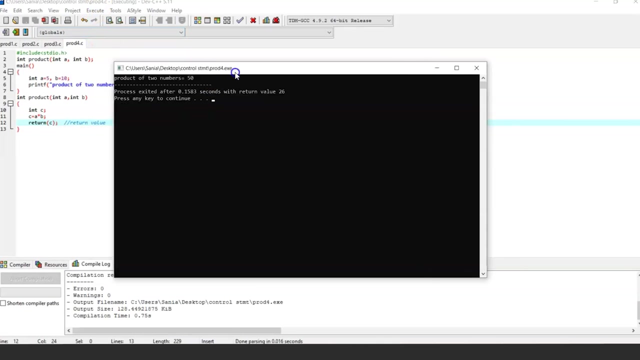 Let's run it. As you all can see, we got an output Product of two numbers is equal to 50.. Last program to execute is function with arguments and return value. Let's run it. so the output is product of two numbers is equal to 50..